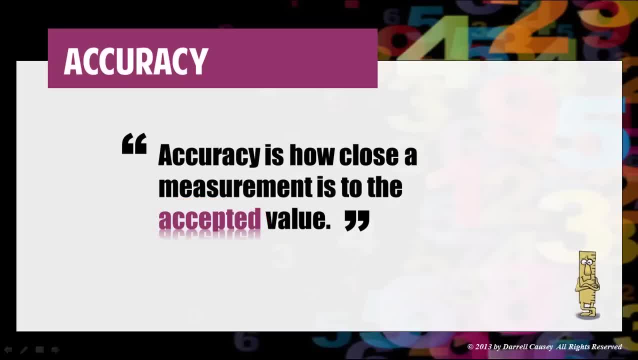 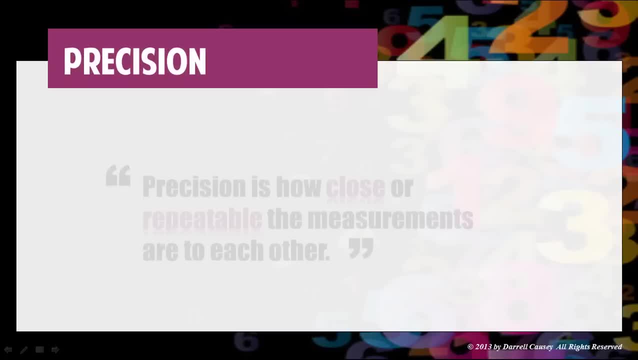 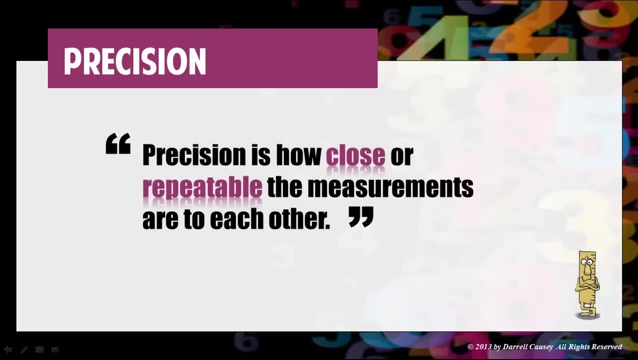 value. Now a lot of people get accuracy and precision mixed up, but this is the definition we will use of accuracy And precision. Precision is how close or repeatable the measurements are to each other. So we have a definition for accuracy and we have a definition for. 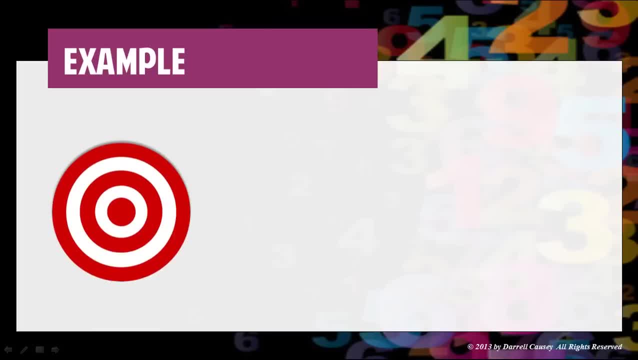 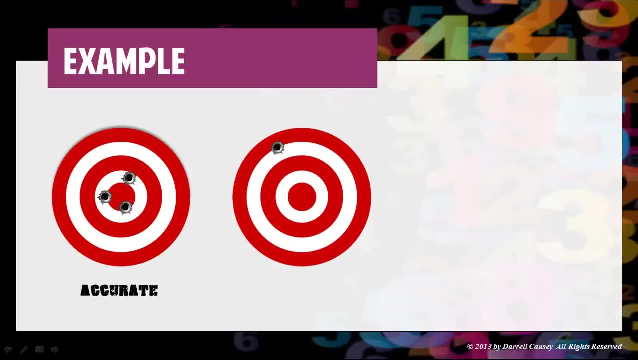 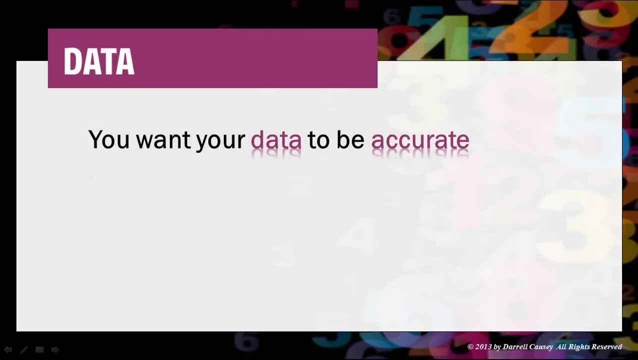 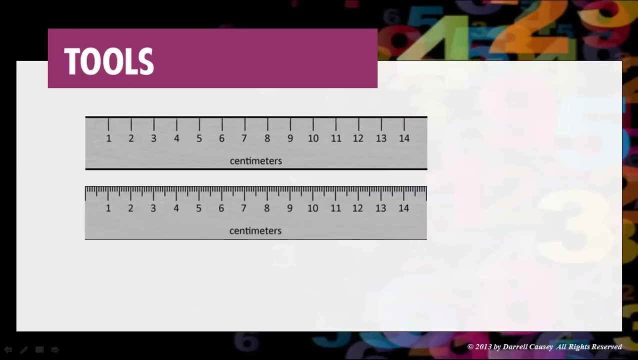 precision. An example: Accurate, Precise, but not accurate. Accurate and precise Data. You want your data to be accurate and precise, As such Tools. A tool is no better than the idiot using it. So let's look. 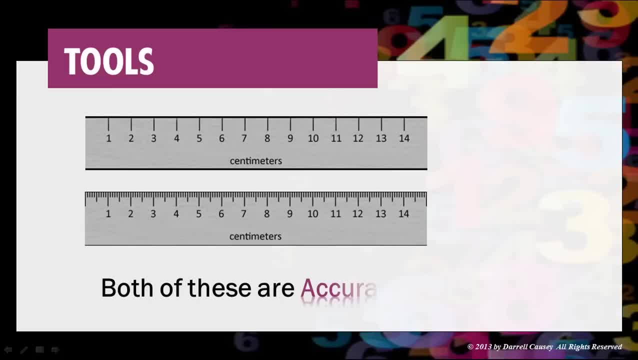 at two tools here. We have the one at the top and one at the bottom. They're both accurate. The bottom one, however, is more precise. You can get a better, more precise and more accurate reading than you can from the top, Or you're going to have to do some guessing. 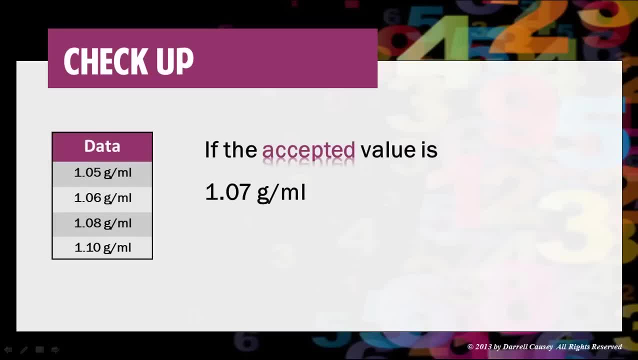 Here's our data. If the accepted value is 1.07 grams per milliliter, The data is precise and accurate. Now look at that data. It is precise and accurate. They're all fairly close to each other and within an accepted value of 1.07.. However, 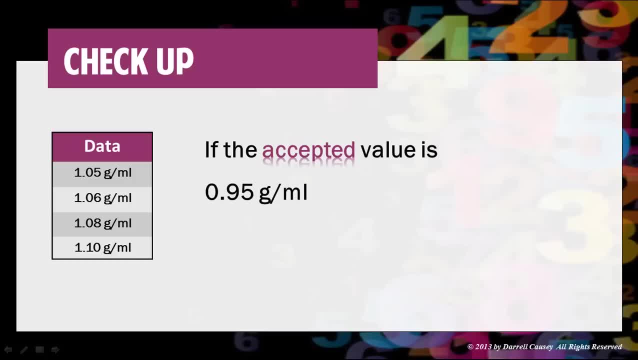 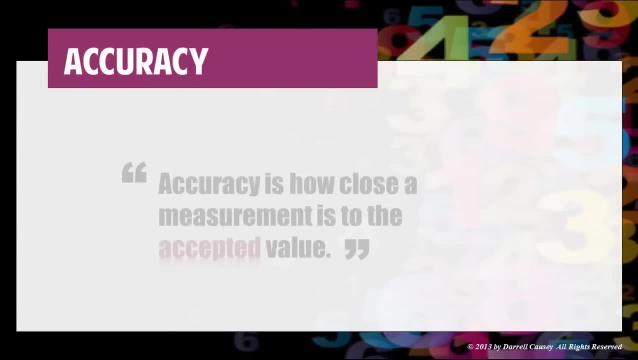 if the accepted value is 0.95 grams per milliliter, it's still precise, but it is not accurate. So accuracy is how close a measurement is to the accepted value, And precision is how close or repeatable the measurements are to each other. 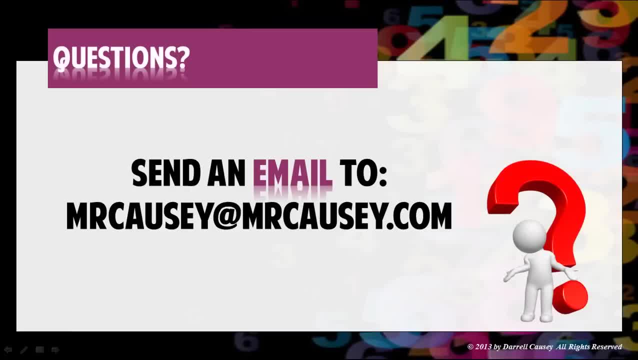 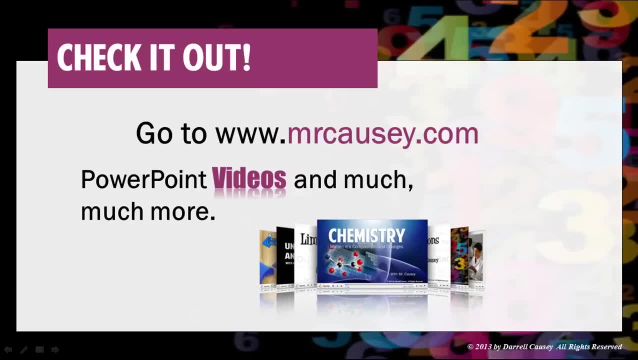 If you have any questions, send an email to mrcausey at mrcauseycom, And be sure to check out mrcauseycom or mrcauseysworldcom for videos and PowerPoints and a lot of information, And be sure to subscribe to my YouTube. Happy IONS everybody.